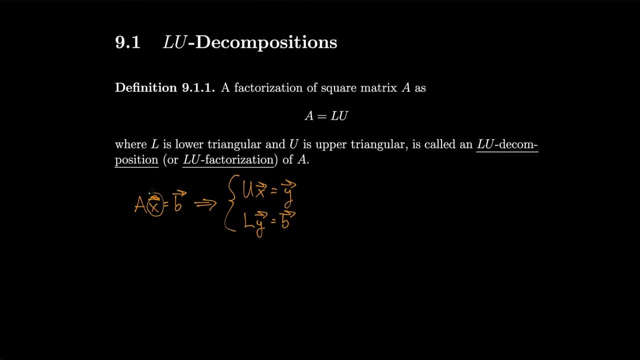 So it gives us an alternative way to solve for X. when we solve systems of equations, We can stop along the way to Y. So the first step to do this is first write LUX equals B, So we just replace A with LU, And then step two is to do the substitution. 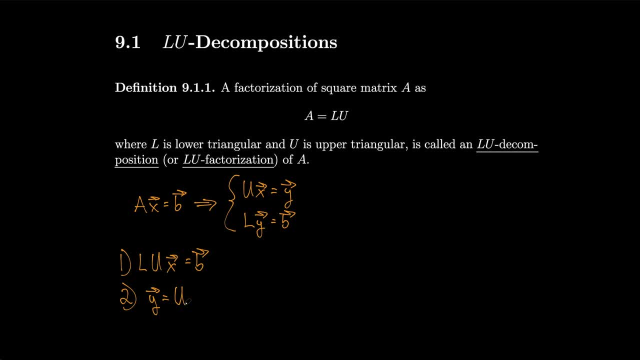 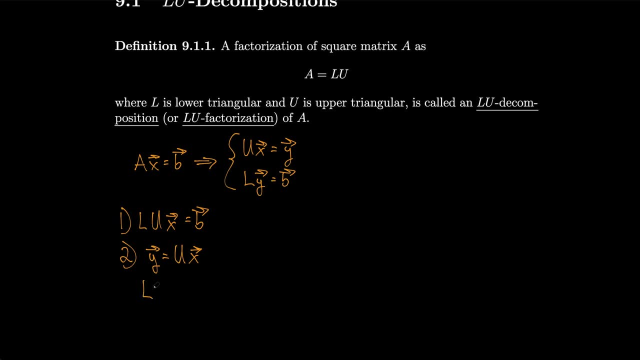 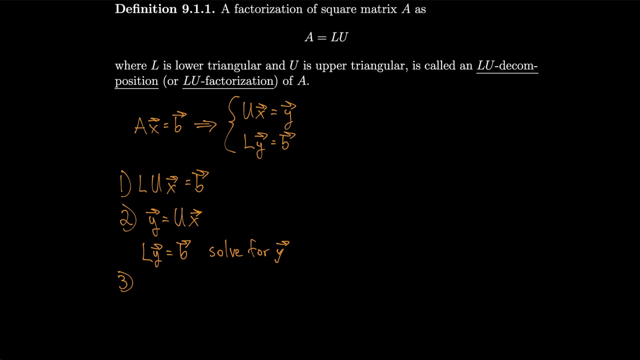 Y equals B And then we'll write: LY equals B, because L times UX is B and we will solve for Y. After we solve for Y, step three is to take what we get from this equation and we'll take what we get from Y from solving this, plug it back in over here and then solve for X. 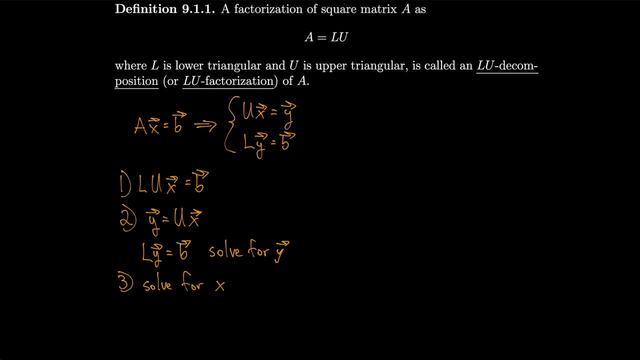 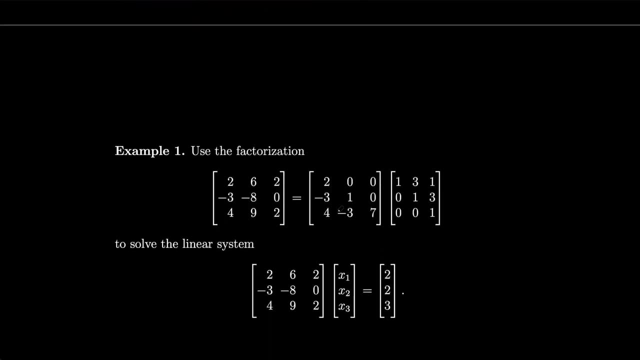 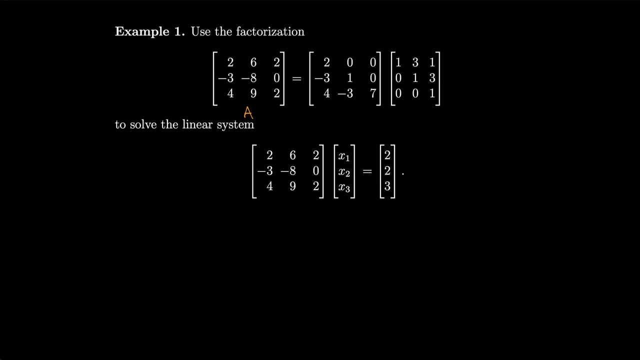 So we don't solve for X immediately, We solve for Y and then we plug that back in and solve for X afterward. Let's do an example of that. Suppose we have this LU factorization right over here. So here's A, here's L and here's U, So A equals LU. 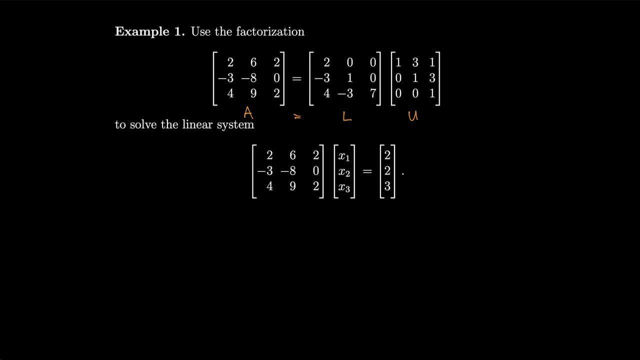 And we want to use this decomposition of A to solve the system A, where the value of X equals B. That's given over here. So Step one, we need to rewrite our system as LUX equals B, So we'll pull off L. so that's two zero zero minus three, one zero four minus zero, so we get. 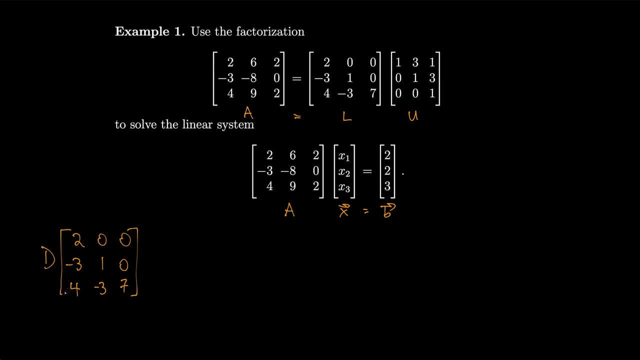 Then we need to multiply by u, so that's 1: 3, 1 0, 1 3, 0, 0, 1.. We then need to multiply by x and set that equal to b, So that's step one out of the way. 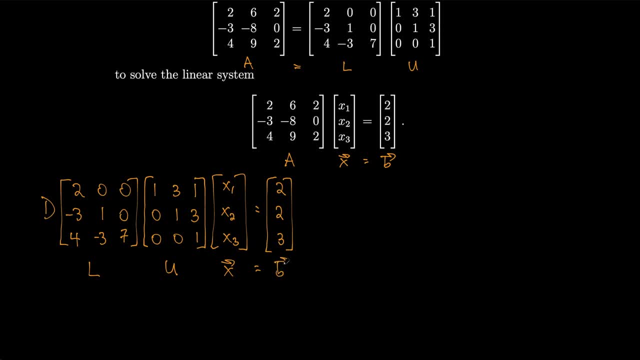 We have l: u x equals b. Now step two is we should write: u x equals y and solve for y. So u is 1, 3, 1.. 0, 1, 3, 0, 0, 1,. we'll multiply that by x and we'll set that equal to y. 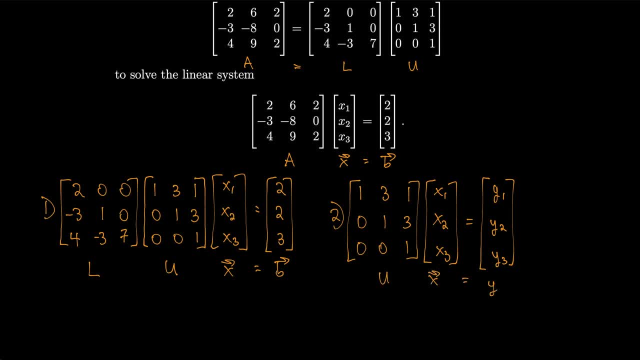 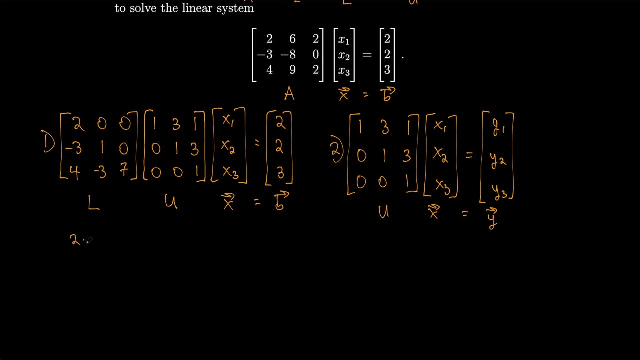 So that's u, x equals y. So now let's solve: l: y equals b For y. so for l we have 2 0, 0, minus 3, 1, 0, 4 minus 3, 7, and multiply that by y. 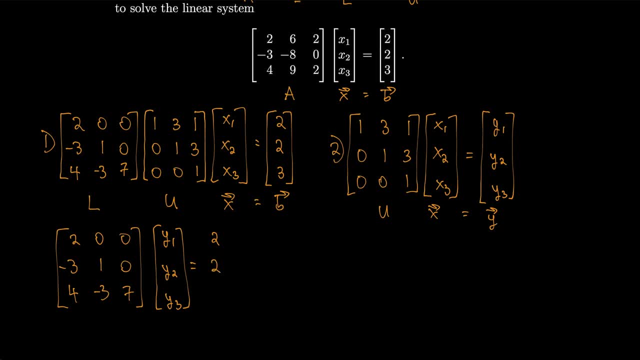 And set that equal to b, So that's l. So l y equals b and this gives us a top equation of 2 y 1 is equal to 2, negative 3 y 1 plus y 2 is equal to 2, and 4 y 1 minus 3 y 2 plus 7 y 3.. 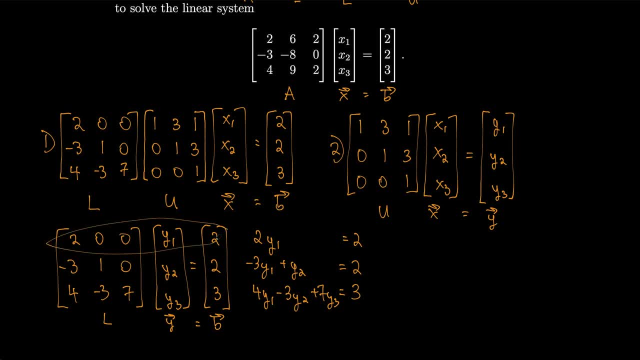 So that's l: y equals 3.. All I did was read off each of the rows. Okay, so that's not a difficult system to solve. because of the fact that l is lower triangular, It makes it much easier. We immediately get that y 1 must be 1, just divide by 2, plug that back in and then. 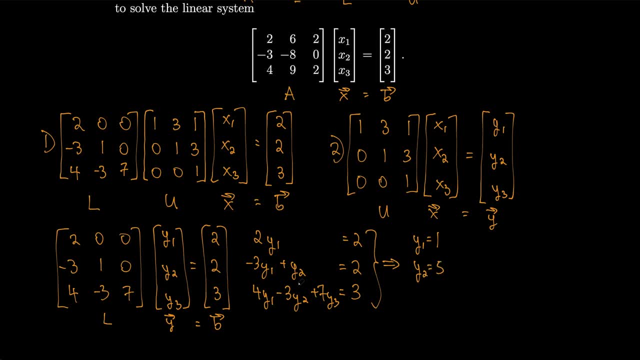 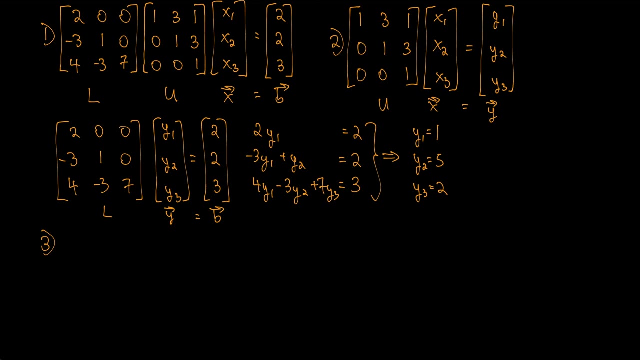 we get that y 2 is 5, and plug both those into the bottom equation and we get y 3 is 2.. So that's the advantage of the decomposition is that it's easy to solve for y. So now we can go back in and do step 3, which is now that we have y, we will plug it into. 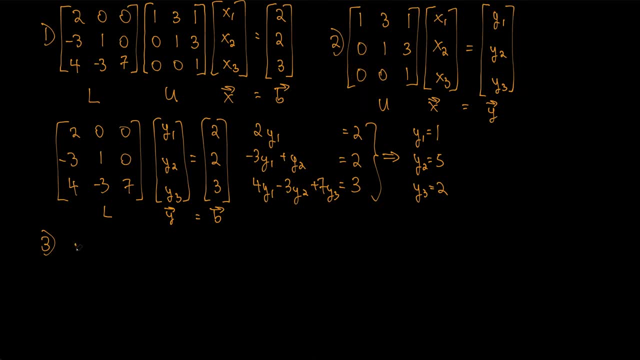 the u, x equals y. equation to solve for x. So we have 1, 3, 1,, 0, 1, 3,, 0, 0, 1, multiplied by x, And that equals 1, 5, 2, as we now see, because we just solved for all of those y's. 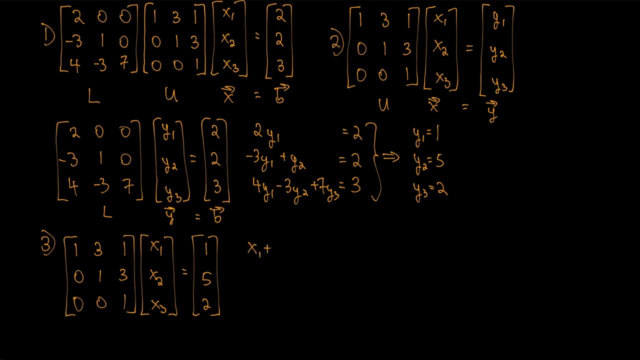 So that gives us a top equation of x 1 plus 3, x 2, plus x 3 equals 1.. Just by reading off that row. Second equation: x 2 plus 3, x 3 is equal to 5. And x 3 is 2.. 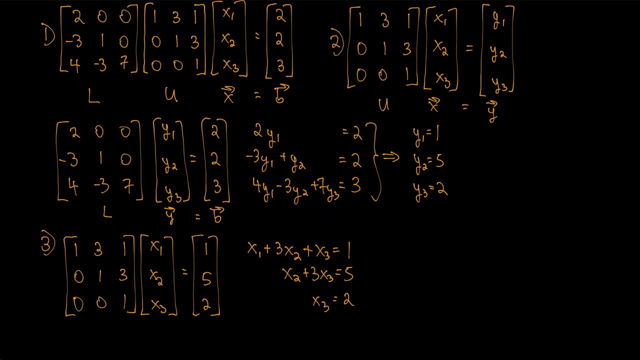 And just like it was easy to solve this equation because l was lower triangular, it's easy to solve this one because u is upper triangular. We immediately have that x 3 is 2.. And we can plug that back in to see that x 2 must be negative 1, and then plug both those. 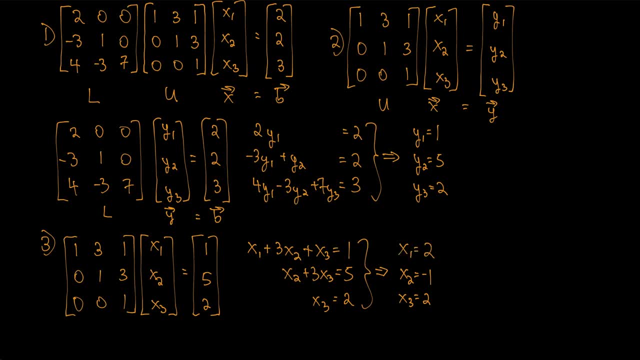 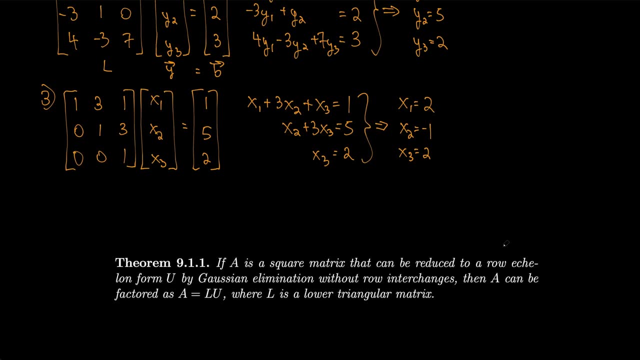 into the top equation to get that x- 1 is 2.. So it makes it pretty easy to solve this equation, even though it may be a little bit tedious to do the split. The hard part really is coming up with the split. a equals l? u. 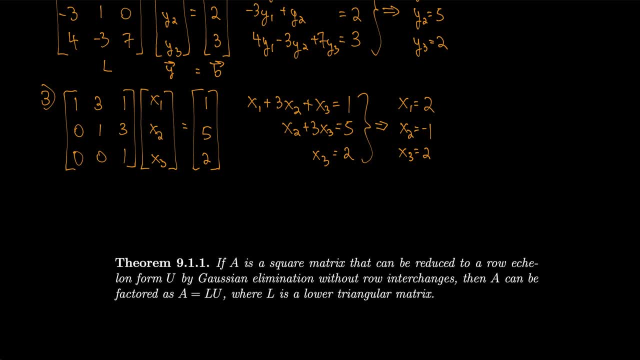 So we have this theorem that if a is a square matrix that can be reduced to row echelon form u by Gaussian elimination without any row interchanges, then a can be factored as a equals l? u where l is a lower triangular matrix. 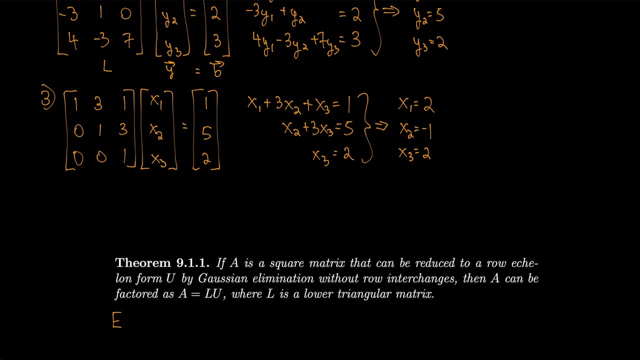 So it's not super difficult to see why this is true If we were to write e k times e k minus 1, et cetera until you get to e 2, e 1 times a. all of these elementary 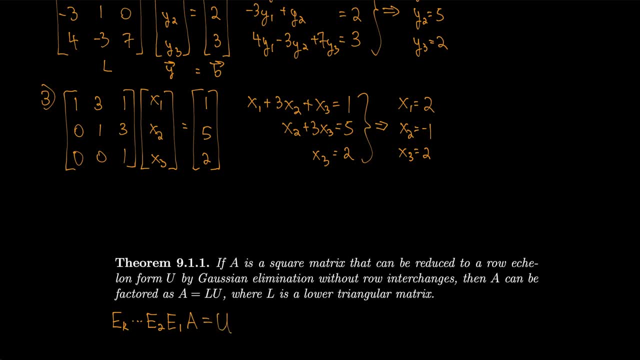 matrices times a equal to u. So if a could be reduced to row echelon form u by Gaussian elimination, then we'd be able to write a equals e, 1 inverse e 2 inverse through: e k minus 1, e 2 minus 1, e k minus. 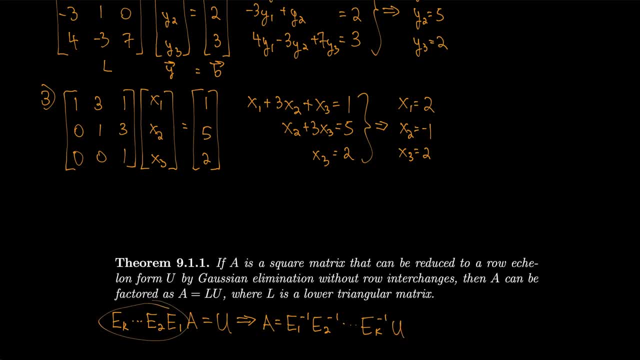 1, e, 2, inverse u. All these e's are lower triangular, So their inverses are lower triangular And we don't have to worry about them breaking that lower triangular nature because we know that we don't have any row interchanges. 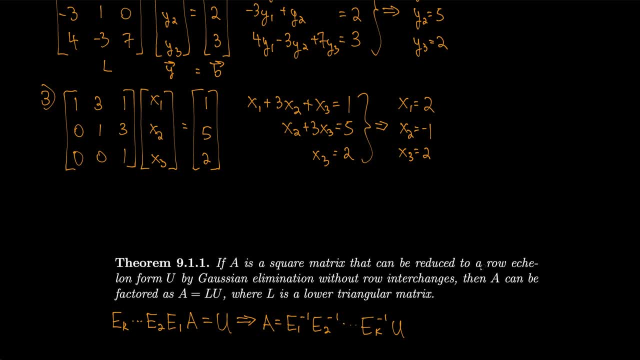 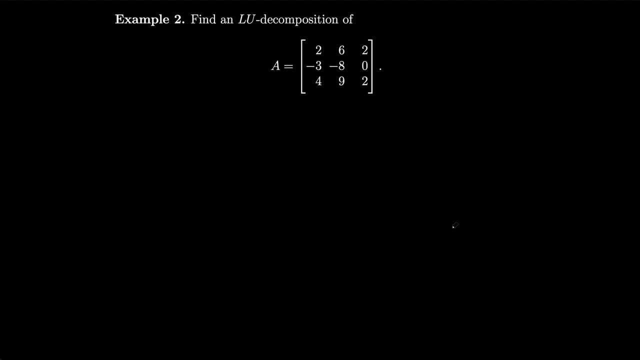 So they couldn't have swapped and moved around anymore. Let's take advantage of this theorem and find an LU decomposition of this matrix right over here. So what we have to do is we have to reduce it And keep it. So I'm going to do it. 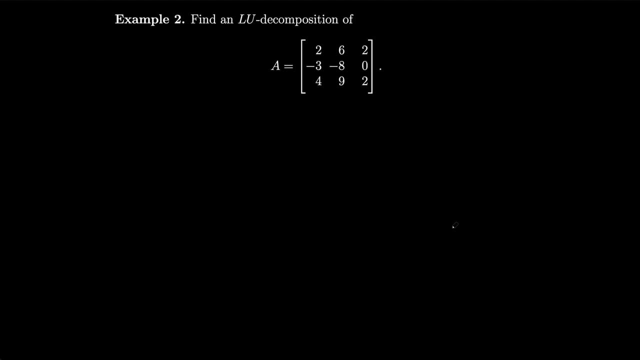 I'm going to keep track of the elementary matrices we're using and their inverses. So it's not super easy. Let's start by taking half of this first row. That way I can get a leading 1.. So I'll make the top row 1,, 3,, 1, and keep the other rows the same. 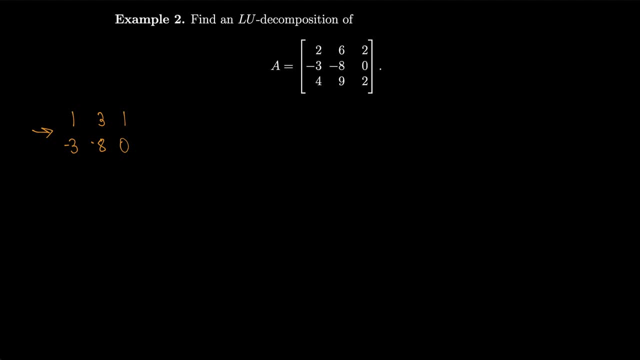 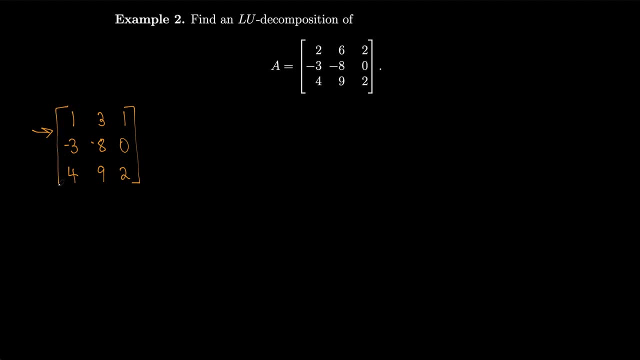 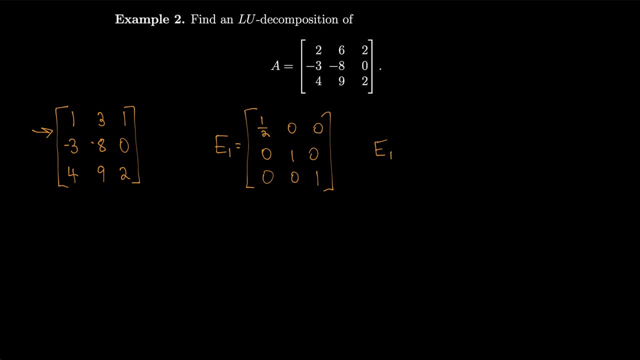 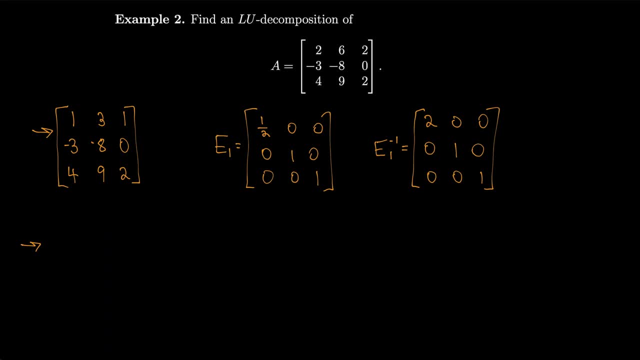 We want to keep reducing it. So how about I get a 0 underneath the 1,? so I'll have 1, 3, 1.. 0, 1, 3, 4, 9, 2, because I'll just take 3 of this first row and add it to it. so that means 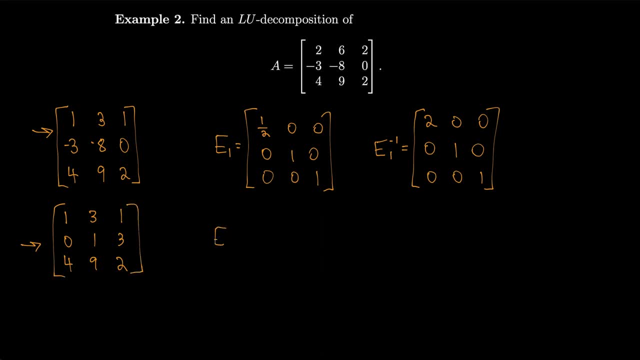 that my elementary matrix that does that should be well the same for the top row. I didn't modify that. I'm just taking 3 and adding it, so I'll just have a 3 over here. okay, so that means that the inverse of adding 3 would be subtracting 3, so I have 1, 0, 0 minus 3. 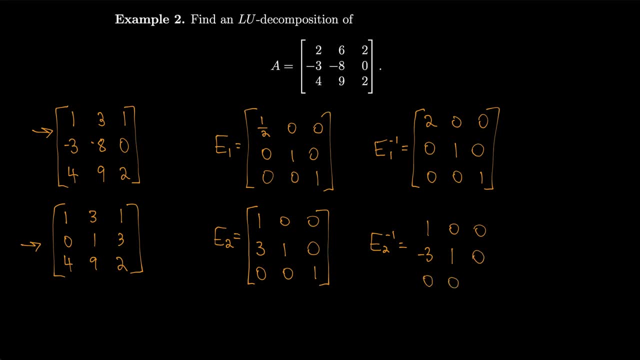 minus 3, so that means that the inverse of adding 3 would be subtracting 3, so I have 1 0, 0 minus 3, 1 0, and you can either multiply this by e2 to convince yourself: it's the inverse. 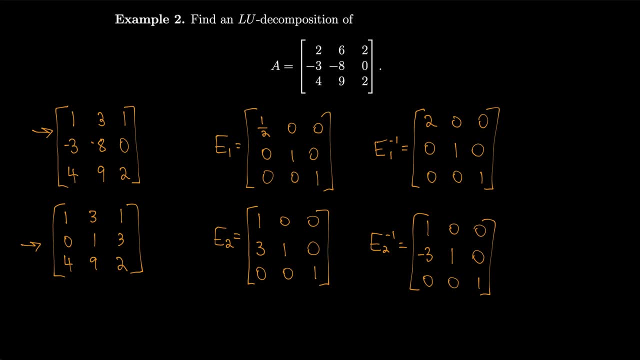 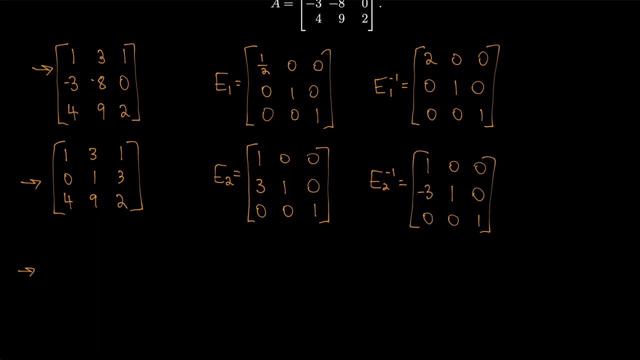 or you could take the inverse of e2 and come up with this. in any case, let's keep going, let's keep reducing. so I need to get another 0 underneath, so I'll keep my top two rows the same and I'll end up with 0 minus 3 minus 2. 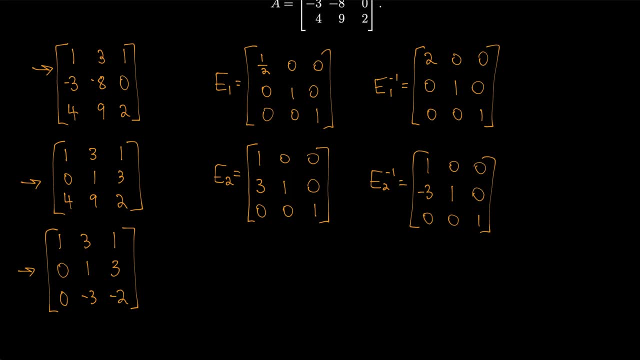 by subtracting off 4 on the bottom. so e3 will be 1 0 0 0, 1 0 minus 4 0 1, which means that e3 inverse is 1 0 0 0, 1 0 4 0 1. 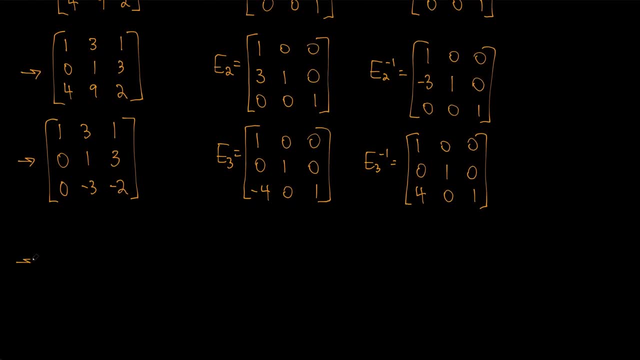 okay, almost there. how about I write- let's see: 1, 3, 1. that's fine, but I need to get a 1 in the second row. I already have it great, so I need to get a 0 underneath it. so I'll write 0, 1, 3 and 0 0, 7, because I'll just take 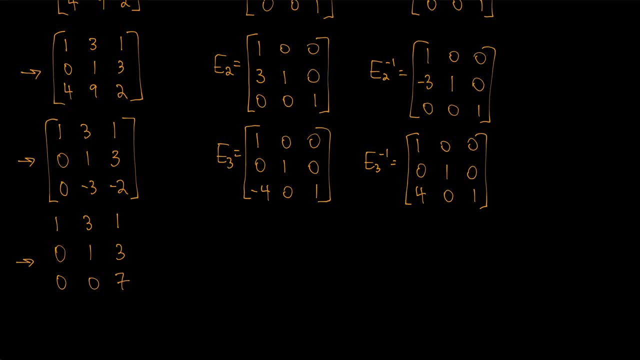 0 1 3 and 0 0 7, because I'll just take 0 and 0 0 7. because I'll just take 0 1, 3 and 0 0 7, because I'll just take a 3 of this row and add it to it. so that means that e4 is 1 0 0 0, 1 0, 0, 3, 1 okay. 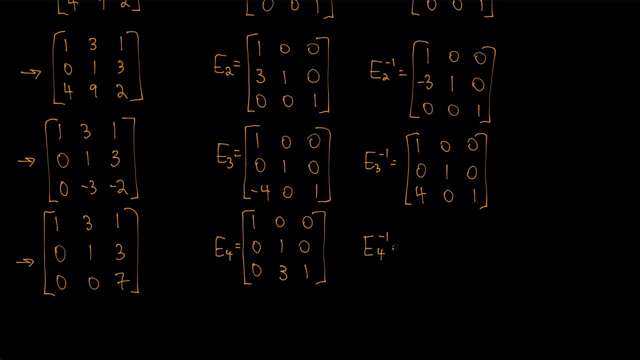 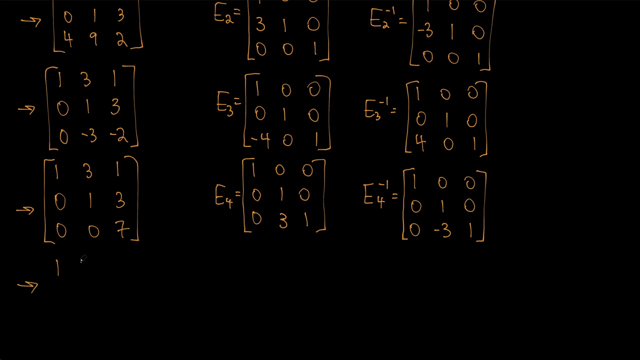 so e3, e4, inverse- sorry- is 1 0 0 0, 1 0 0 minus 3, 1. okay, almost there, we have still 1, 3, 1 is fine, 0 1, 3, and then I just need to get a 1 over there and then this thing will be upper. 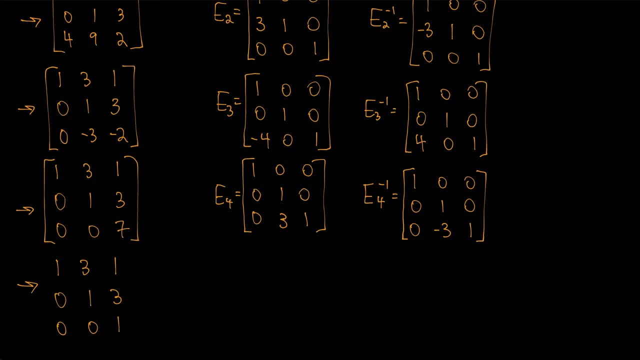 triangular, so 0 0, 1. all I have to do is multiply by 1- 7th, and then there we go. this is an upper triangular form that could be our U, so that makes e5 equal to 1, 0, 0, 0. 1, 0, 0, 0, 1, 7th. 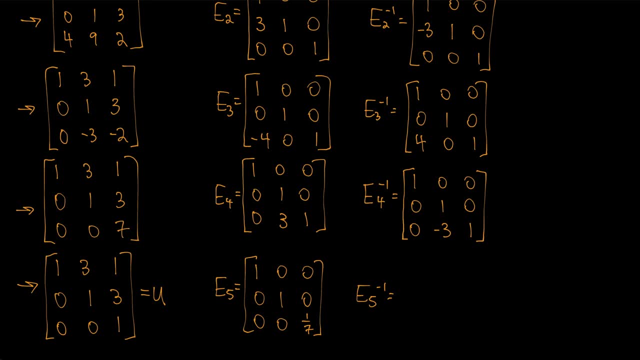 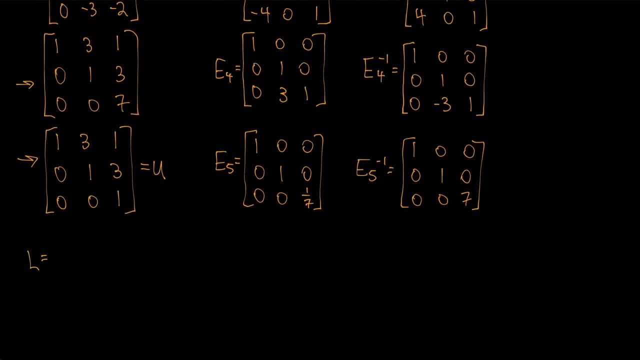 and thus e5 inverse is 1 0 0 0. 1 0 0 0, 7. okay, that gives us L. so now we have that. L is just all of these e inverses multiplied by each other. so I have 2 0 0 was our first one- 0 1 0 0 0. 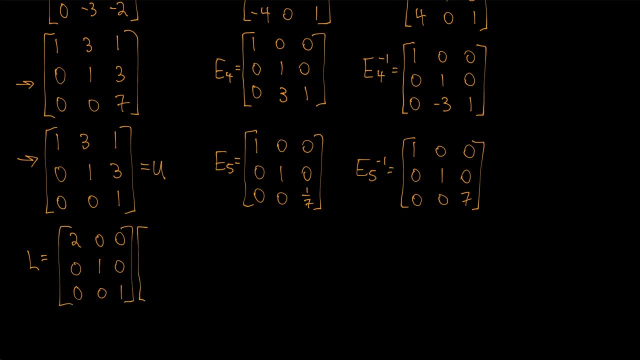 1 multiplied by 1 0 0 minus 3: 1 0 0 0, 1. that was eat u inverse and now e3 inverse was 1 0 0 0, 1 0, 4 0, 1 and then e 4 inverse: 1 0 0 0. 1 0 0, 1 0. 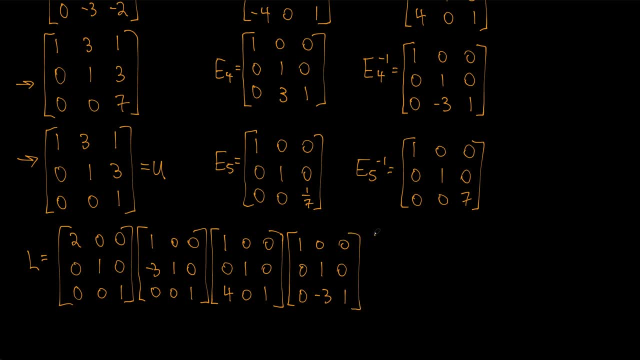 0, minus 3, 1, and last matrix to multiply by 1, 0, 0, 0, 1, 0, 0, 0, 7.. And if we do all the multiplication, we get 2, 0, 0, minus 3, 1, 0, 4, minus 3, 7.. 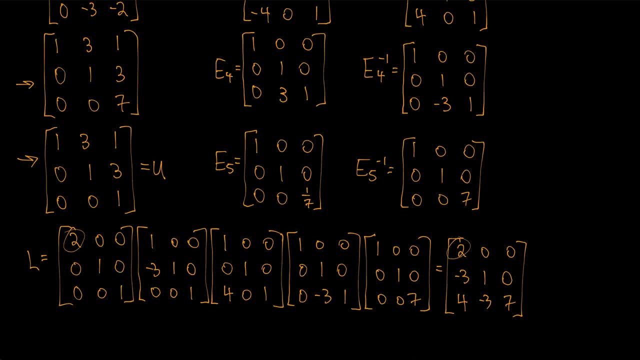 And notice that all you have to do is take the 2, take the minus 3,, take the 4, the minus 3, and the 7.. So it's an easy multiplication to do. So that means that we have our LU decomposition. 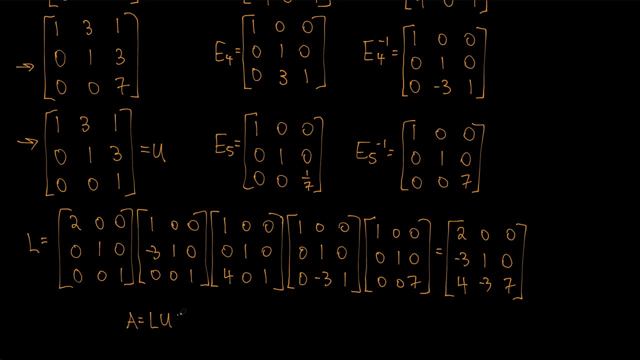 We have A equals LU is equal to 2, 6, 2.. Minus 3, minus 8, 0, 4, 9, 2.. Equals- sorry, that's A equals- 2, 0, 0, minus 3, 1, 0, 4, minus 3, 7.. 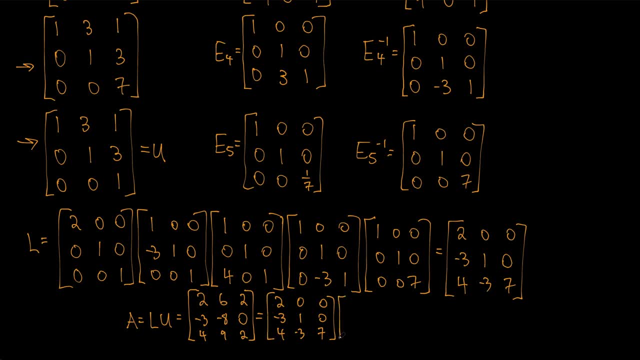 That was our L And U. we reduce. We reduce to 1, 3, 1, 0, 1, 3, 0, 0, 1.. So, yeah, it's way easier to solve for x when you already have the LU decomposition. 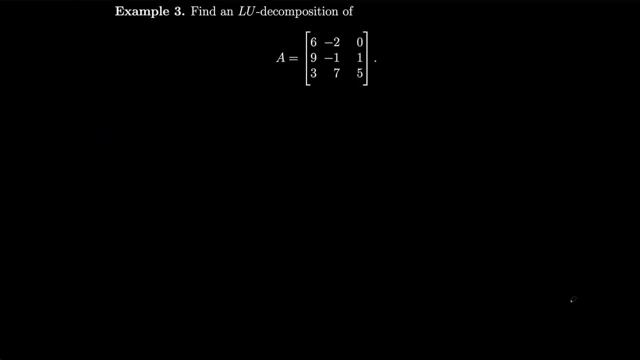 Let's do one more example and find the N? LU decomposition of this A right over here. What we can do, instead of writing out E and E inverse every single time, is we could just write out a lower triangle. And if we have the lower triangle now that we gotta keep track of each of the missing numbers that appeared in L. 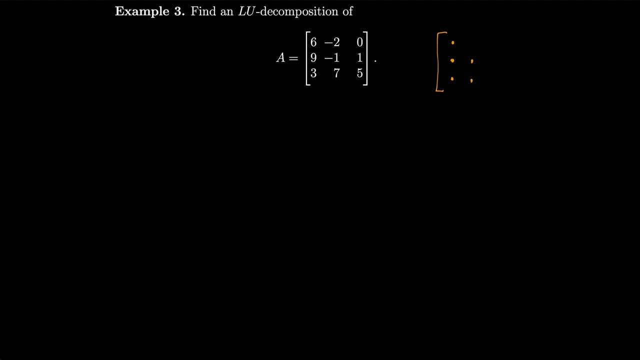 which we found was just a part of the entire matrix, Now that we saw that each of those numbers that appeared in L was just something that we could have obtained by keeping track of the operation that we were doing. Remember, it has to be lower triangular, so all these guys have to be 0. 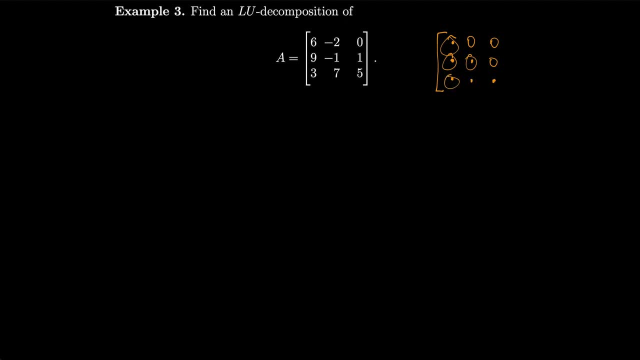 If we keep track of each of these missing numbers in our matrix along the way, then we don't have to write E and E inverse every single time. We could just build it, So let's do that. See how easy that was. You get the question. 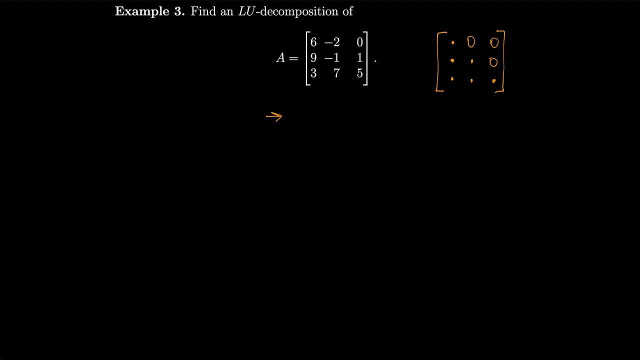 Yeah, So let's first start by taking 1 sixth of that, so 1 minus 1, third, 0, and the second row is 9 minus 1, 1, not changing it yet- and we have 3,, 7,, 5.. 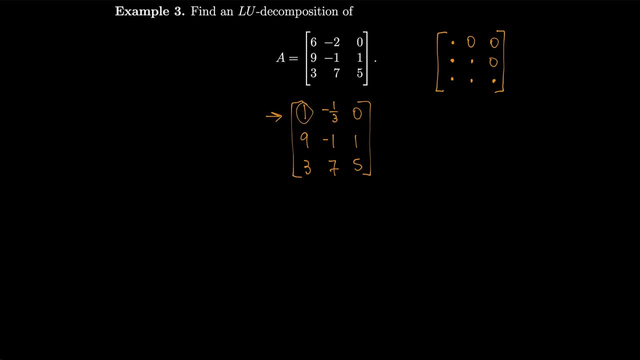 So what I did here was I took 1 sixth of that. so that means that the inverse would have a 6 in it. so I could just put a 6 in For that dot And then the other ones. I still don't know yet. 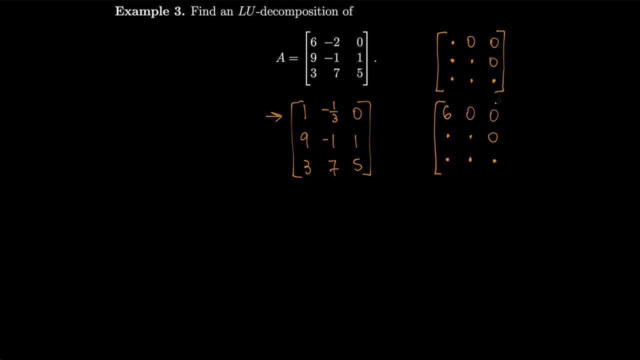 So I'll just fill those in, and I still have my zeros, So you can just fill it in dot by dot and then you'll build your L. Okay, so let's keep going. So I have 1 minus 1 third 0, not touching the top row now. 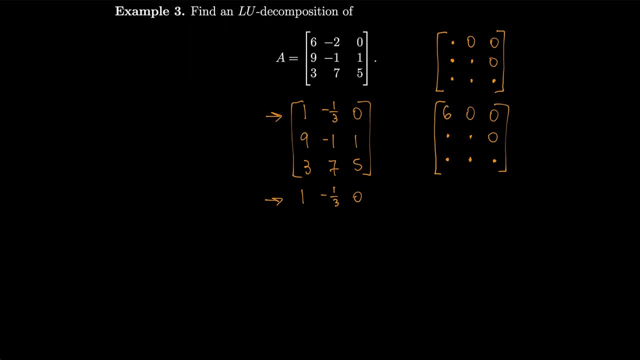 I'll subtract off 9, so I'll have 0,, 2,, 1,, 0,, 8,, 5.. I can do both of these at once, right as long as I keep track of both dots. So for this one I needed 9 to be subtracted, so that means in the inverse it'll be positive. 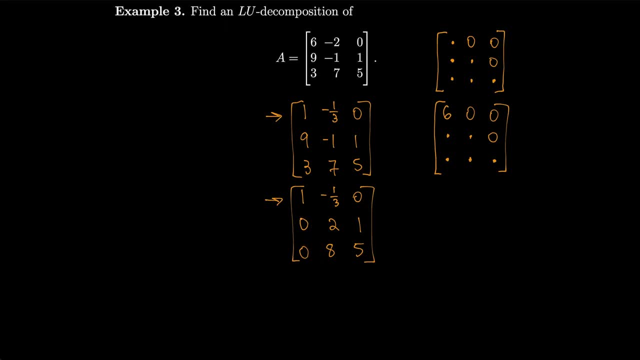 9, and for this one I needed 3 to be subtracted, so in the inverse it'll be positive 3, so I filled in 2 of the dots. So I have 6,, 9,, 3, and then I just have 3 dots left as my placeholders. 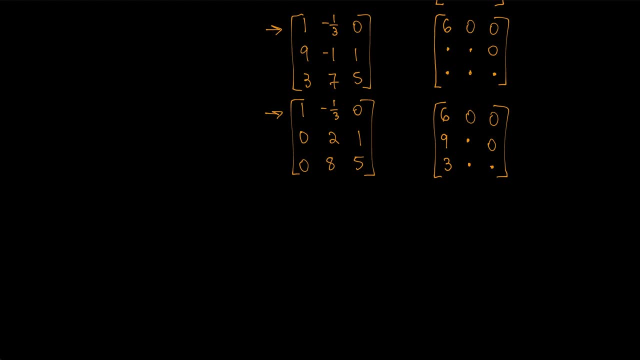 Okay, getting there, Let's do our next step and we'll get a 1 over here instead of the 2, so we just have to divide by 2.. So let's do that: 0, 1, half and 0, 8, 5.. 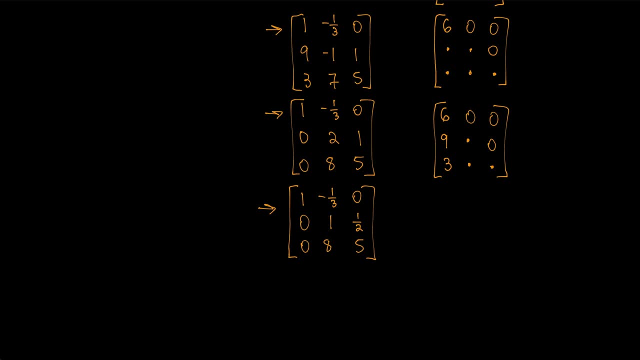 Okay, so dividing by 2 means that the inverse would be multiplying by 2, so I have 6, and 9, 3 still, but now I have a 2 over here for this dot. we just have 2 left to figure. 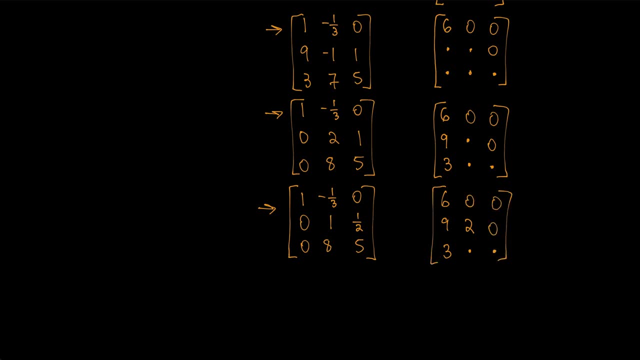 out Okay. so I've got 1, and I can sit there at 0 still. I have 0,, 1, half still. let's see if we can get a. how about a 0 over here and I can get a 1 over here?